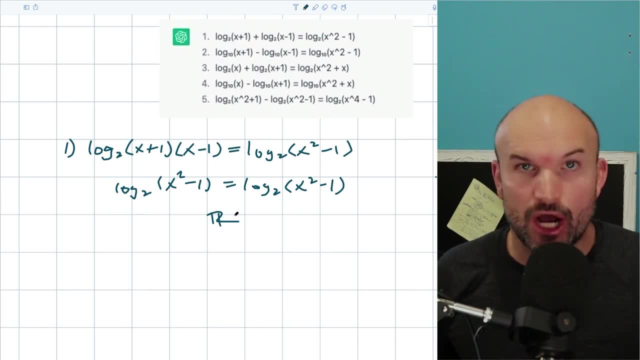 something wrong. right, And of course I could be, but it looks like to my case the solution is going to be all real numbers. Um, not X. X is equal to two, So um, looks like we need to let the AI know about that and it's going to get. 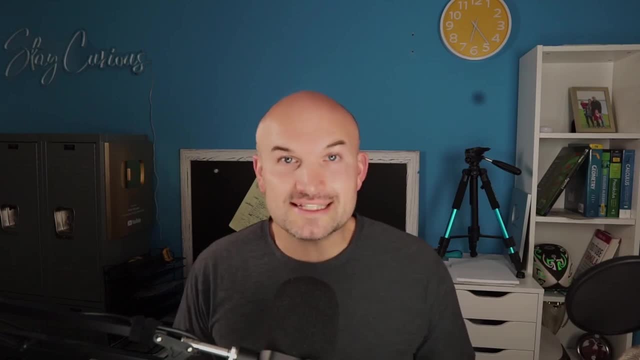 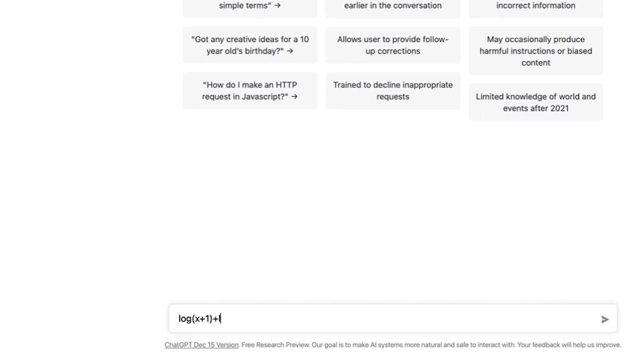 smarter And, I think, eventually write all of its wrongs. So since they got it wrong, let's go and type in exactly what this equation is, to see if GPT does any better. So type it in the original equation. Now, in this case, I'm not going to use base two, I'm just going to use regular log. 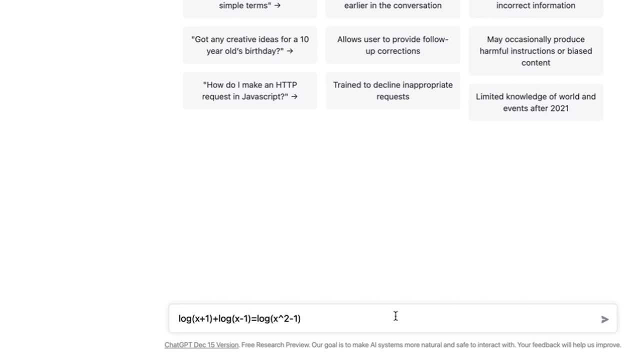 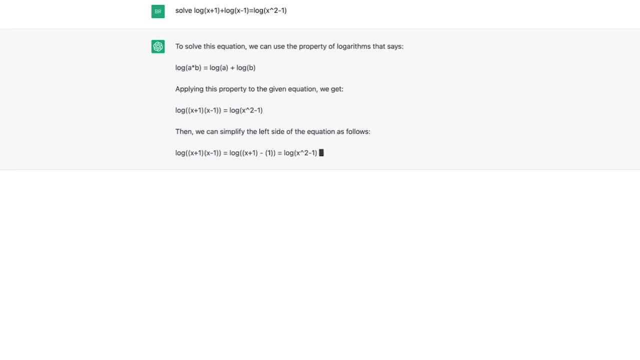 because I use the one-on-one property anyways, So it doesn't really matter. Okay, So now that I go ahead and typed it in, let's go ahead and see what's the- and actually you know what let's type in. let's say: solve this, please. Cool, So you can see. actually. 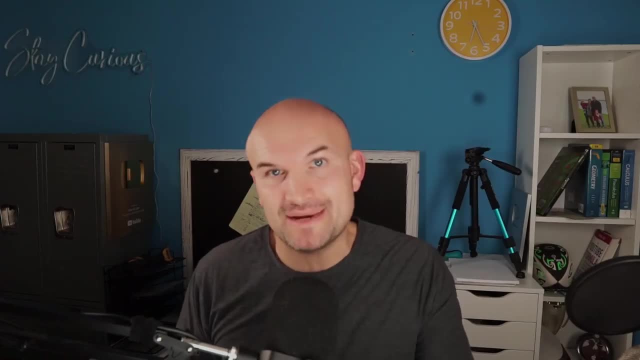 that it worked out correctly and myself I can kind of follow through with this step-by-step process. So it didn't get the right answer initially, but when I was more specific on what I wanted it to do, it looked like it redeemed itself All right As an example. 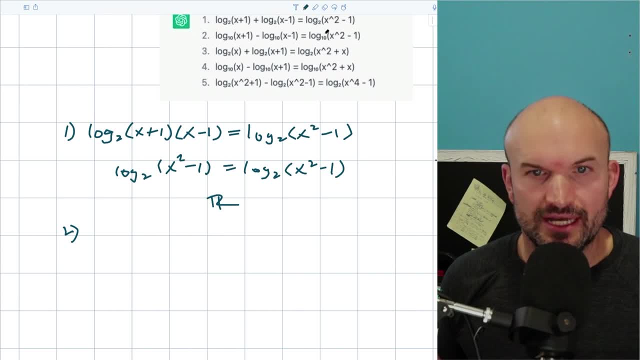 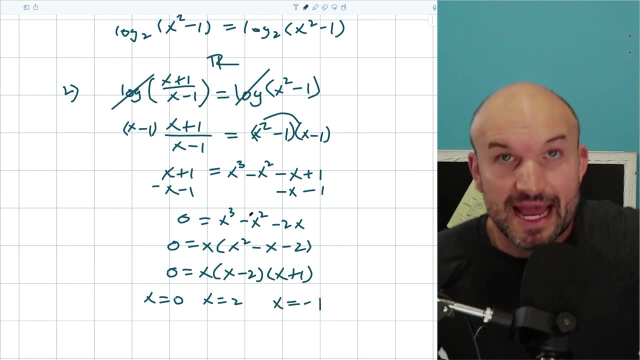 we have X base 10 of X plus one minus an X. base 10 of X minus one is equal to an X squared minus one. So now, using the zero product property, I can say: X equals zero, X equals two and X equals a negative one. So now let's go back and test to see right. We want to look for extraneous. 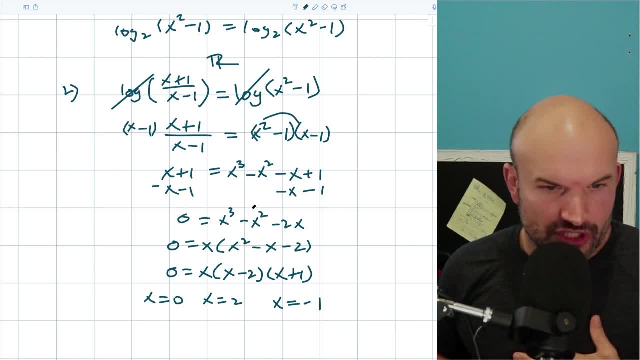 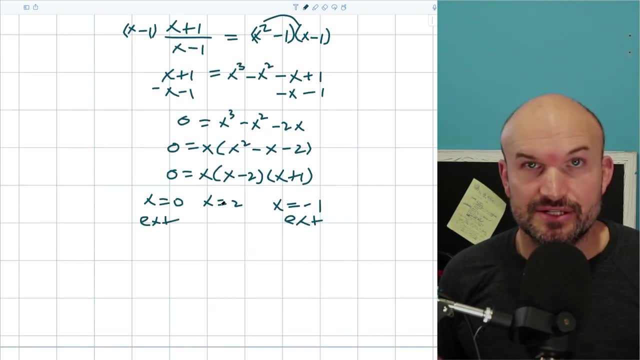 solutions, because when we're dealing with logarithmic equations, just because it solves this quadratic here, if it doesn't go back and satisfy the original equation, then it's an extraneous solution. These two answers are extraneous, So the only answer is: X equals. 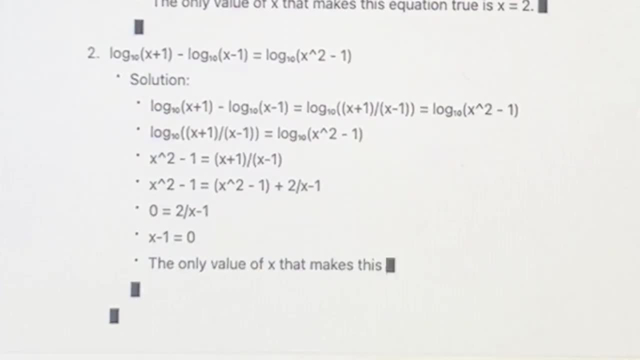 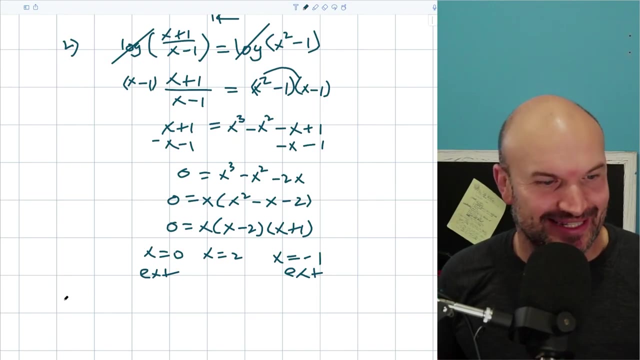 two which go ahead and taking a look at my original screenshot. original answers. X is equal to one, which is not even an answer I got. So not sure what's going on here, but I'm pretty sure my answer, everything that I did, is correct. So again, it got it wrong. 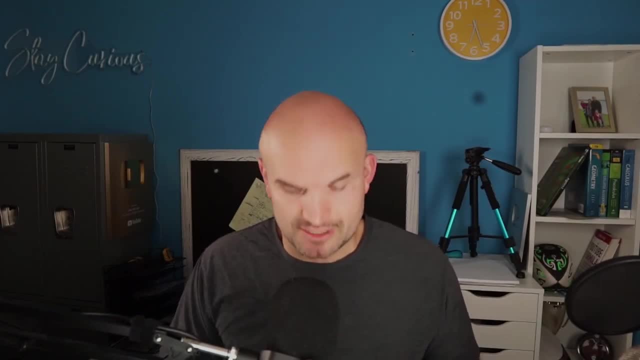 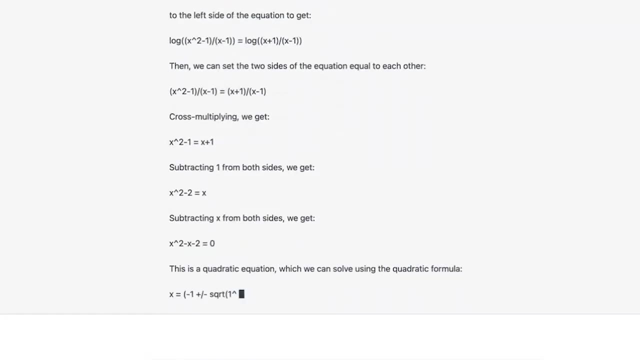 So now I want to do is plug it directly into chat GPT and see how it works. Okay, now, in this case it is not getting the same answers, And if you look at this quadratic, the X squared minus X minus two equals zero. Like the solutions are not negative, 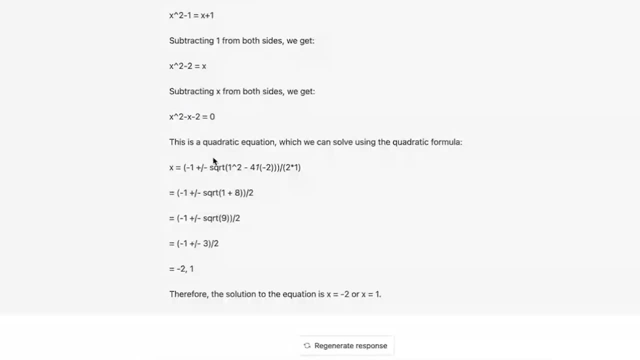 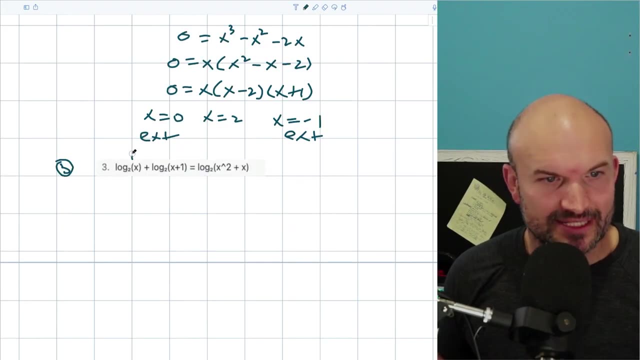 two and one. They should actually be a negative one and positive two, And either way those two are going to be extraneous. So in this case we can see that is failing us again. Let's maybe go ahead and try number three. So we have these two arguments they have. 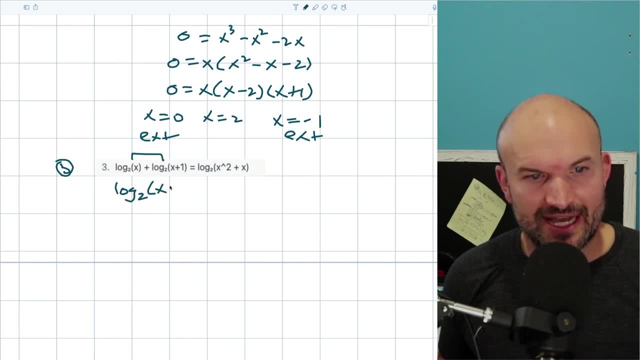 the same base, right? So I can just rewrite this as a log base: two of X times X plus one, And that's going to be equal to a log base two of a X squared plus X. So again, this is going to have all real numbers as its solution. 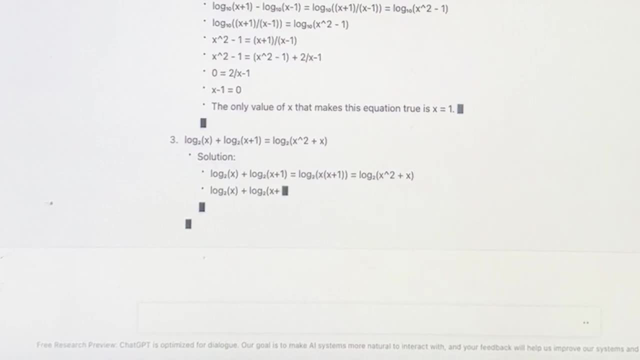 Not really sure what the algorithm is going And again, if you remember, this is where it started to run out- had a network error. So I'm not really sure what the solution process was for this one. but I'm not getting X equals. 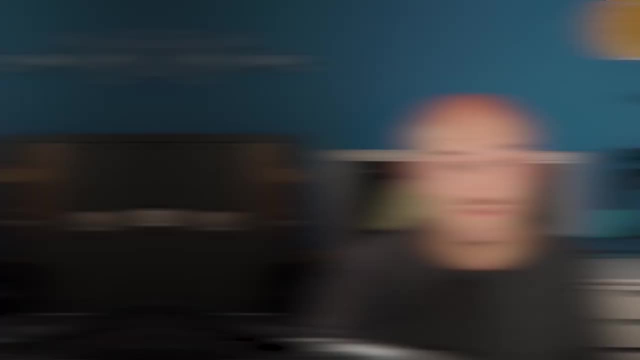 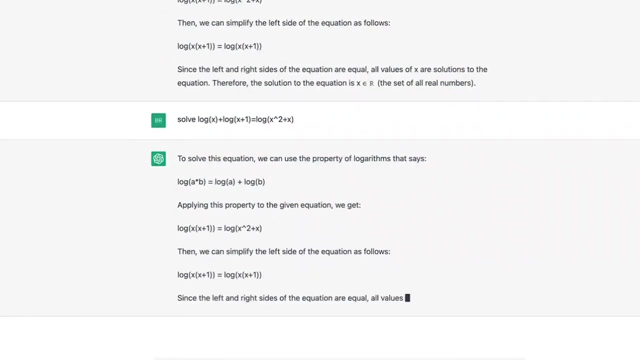 one to be the solution, All right. So right now the AI is not working out so well, So this is again another one where we got all wrong. So let's go and type it in directly and see what it says. In this case, again, it redeemed itself. 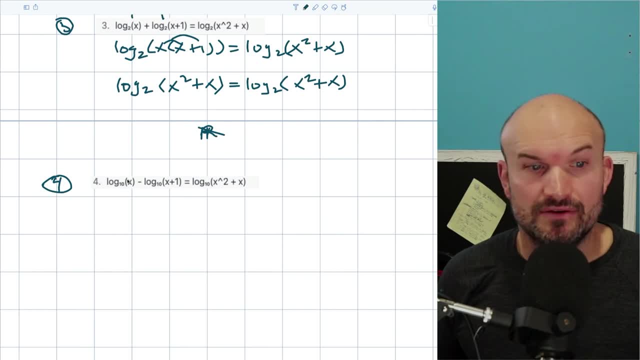 Let's go and try the next problem. Okay, So in this problem we have the difference of these two logarithms. So again, we can rewrite this as a quotient. Okay, So again you can use my one-to-one property. 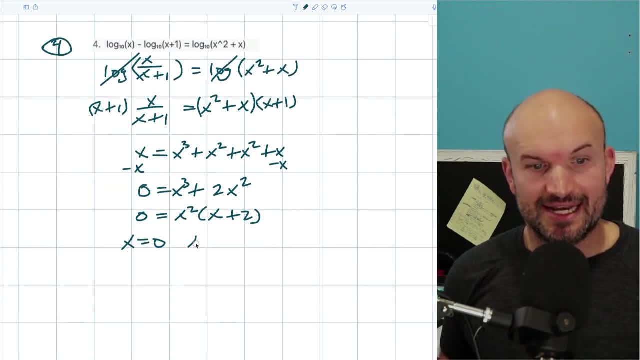 So therefore, using the zero product property, I can say X is equal to zero and X is equal to a negative two. But we, again, we have a problem. I can't plug zero in for X, right, That's going to again be an undefined value. 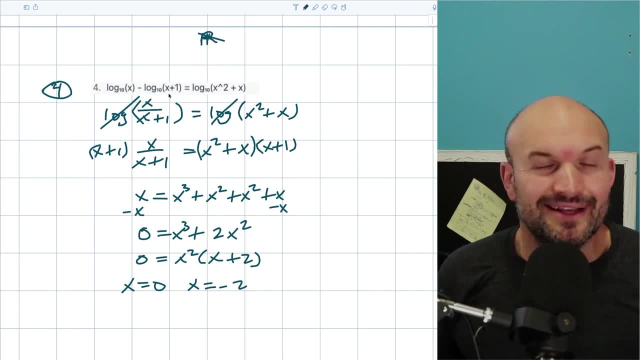 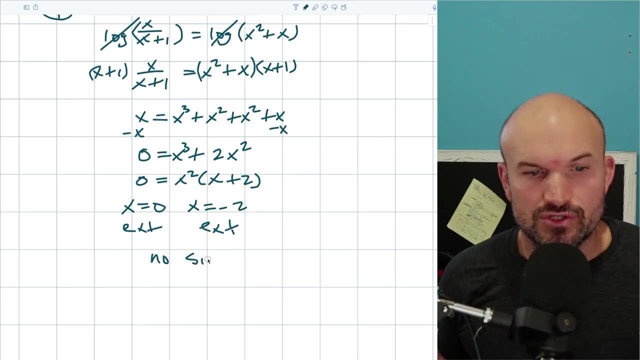 So that's extraneous. And if I plug in negative two, like negative two plus one is going to be negative one. You can't take the logarithm of a negative, So these are both going to be extraneous solutions. So in this example I am seeing no solution. 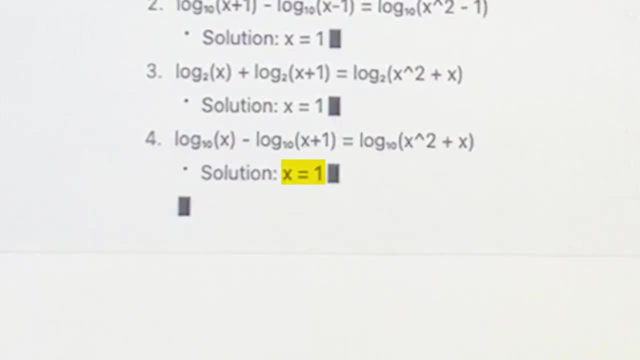 And again the answer they gave us is: X is equal to one, which I am having absolutely no idea how they went ahead and got that All right. Again, we have some extraneous solution, So let's go ahead and type it in and let's see what it says directly. 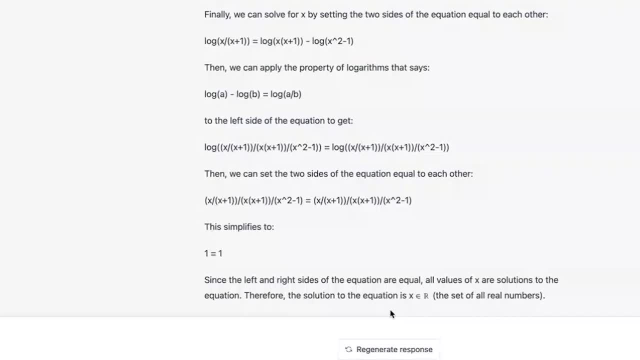 Now, this is not the solution that I got And this isn't the solution that originally got. I also feel like by watching the solution, I just got like kind of overwhelmed, Like this is like a lot going on And it seems like again, we need to give this. 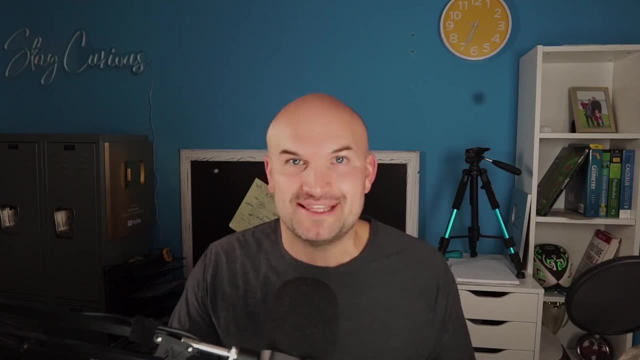 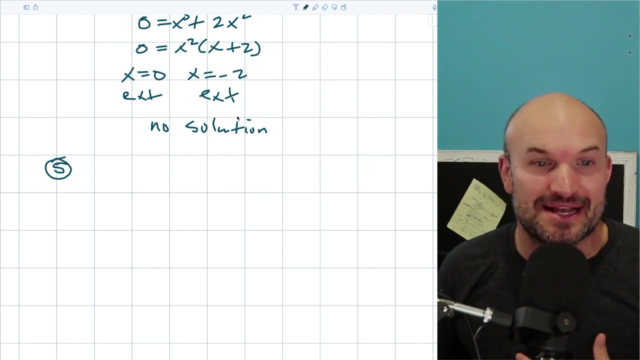 AI a little bit more information and help on solving a problem like this. All right, So I guess there's only one more time to do. Let's try to see if we can get one of these answers Correct, Because so far the problems aren't too bad, but I'm not getting the same answers as the AI. 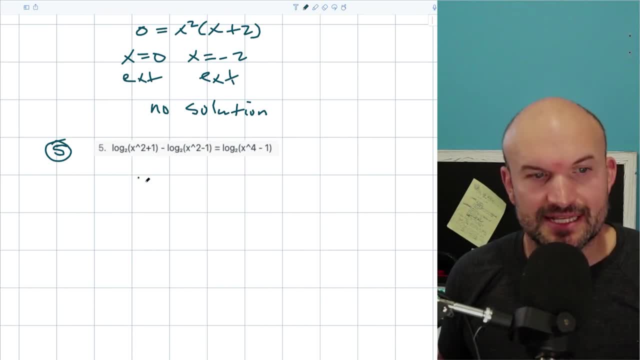 All right. So in this one again we have another difference here, So I can rewrite this as an argument. So, log base two: let's say the quotient here of X squared plus one over an X squared minus one, And that's going to equal a log base two of a X to the fourth minus one. 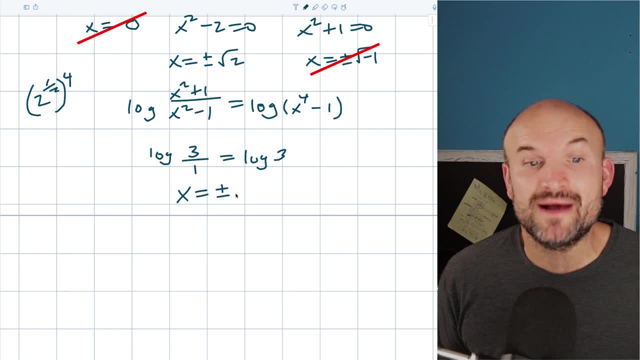 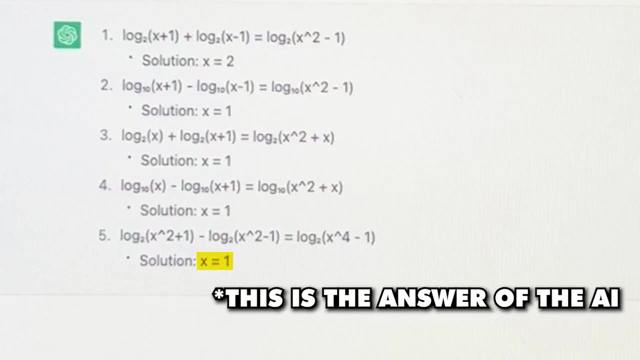 Okay, The solutions to this equation is going to be: X equals a plus or minus square root of two. So, again, if we're going to go ahead and check our answers for what the AI gave us, which is plus or minus square root of two, zero and I, these are going to be our only.